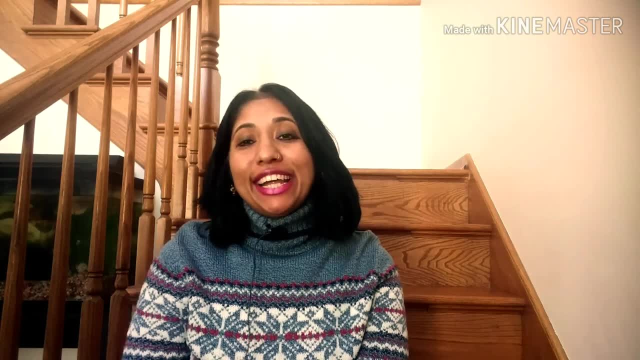 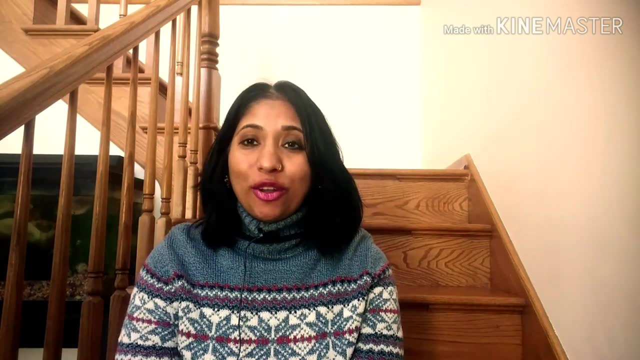 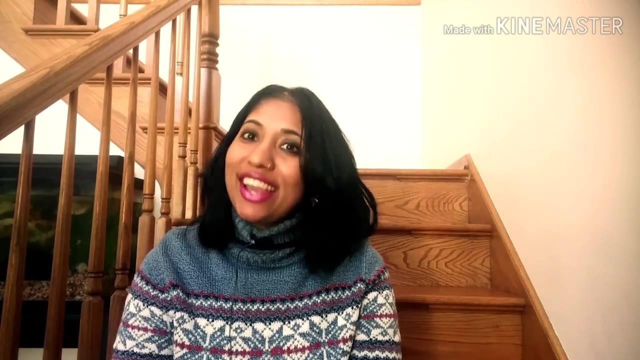 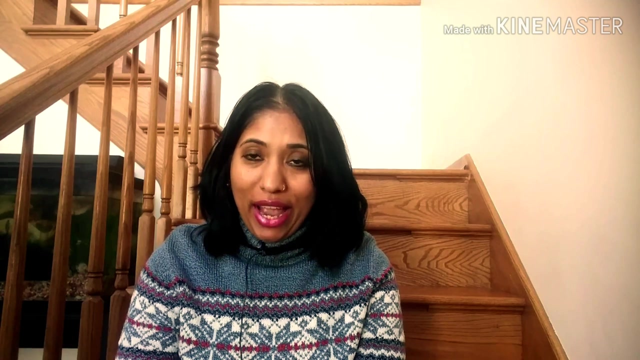 you know, make it more flexible. Western culture people are less conservative. they are adapted to any change. That's one of the thing, because they can adapt to any type of changes very easily. People are more friendly compared to western culture, But, that in mind, eastern people may be less friendly. 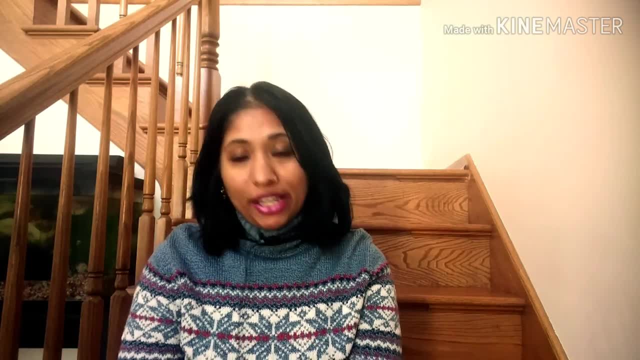 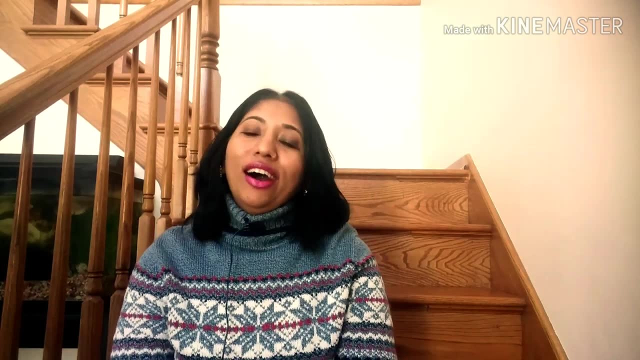 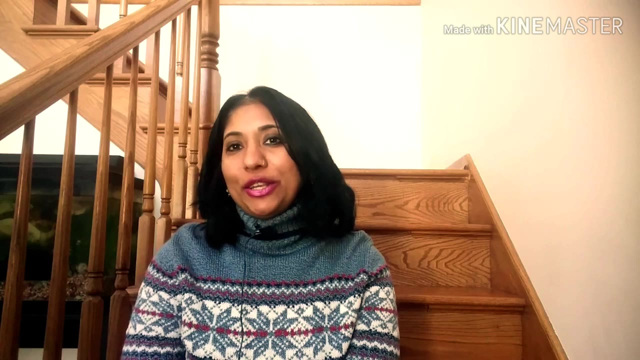 but once they get to know each other they will be friends forever. You know they won't change friends that frequently, like western people. So you know they are not very friendly of friends. but once they, you know, you get to know them, you know, then they are more friendly with you. 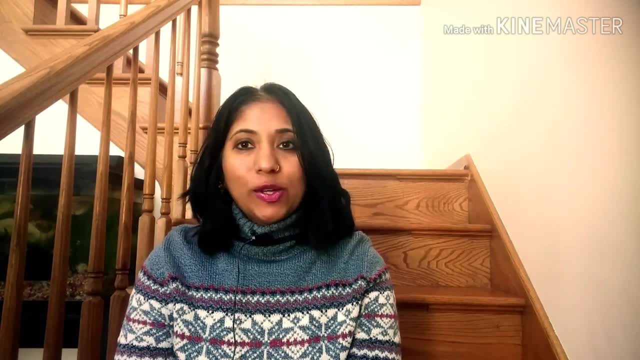 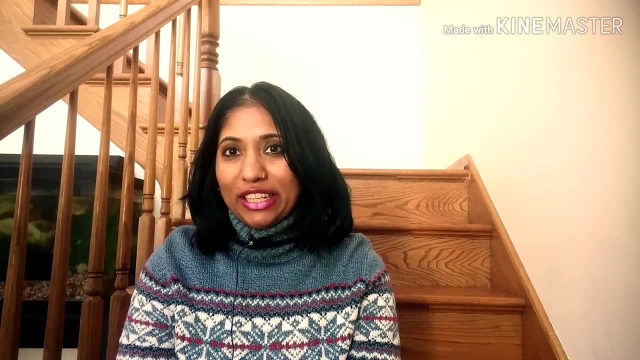 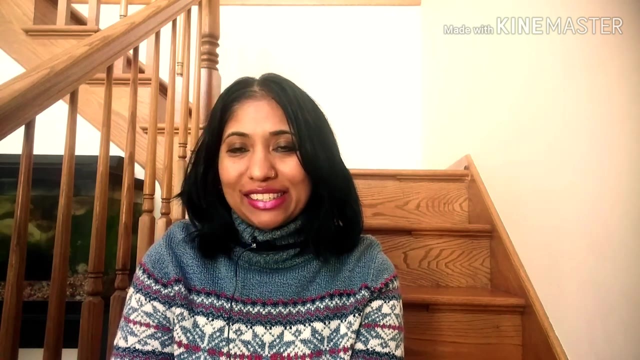 And more genuine with you, You know. so, western people: it's very easy to strike a friendship, but with their differences the friendship can abandon any time. Eastern people: they don't like to mess up their schedule. They are more systematic and more conservative in that way. But western, 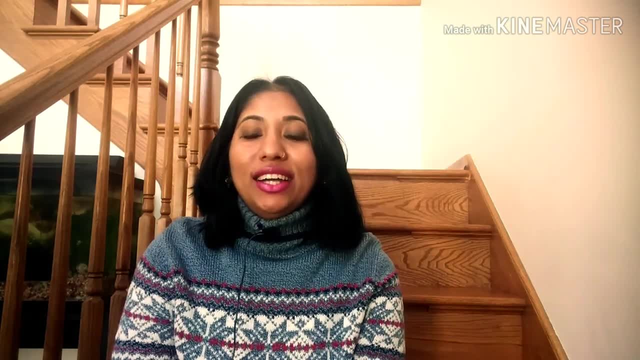 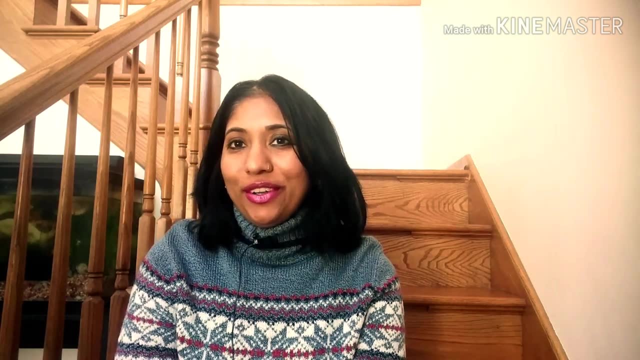 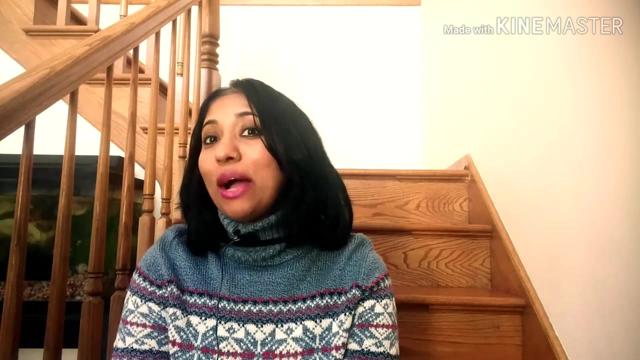 people are more flexible and adaptive way. That's one of the successful thing about the western culture. They will be adapt to, you know, any type of situation. That's why western people are kind of well-leaders compared to eastern people. Another thing, another major difference. 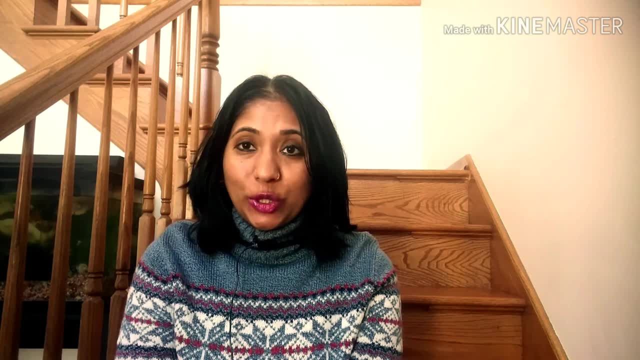 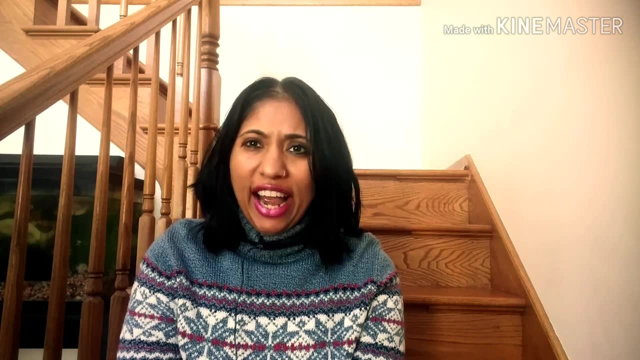 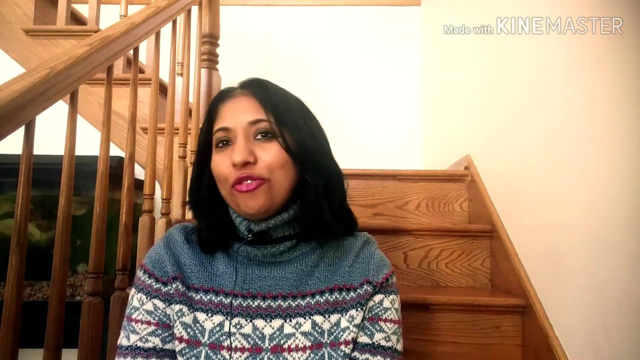 between eastern and western culture is eastern people are more educated. They give more importance to their education. It's very hard to find the eastern person, this degree, They give much importance to education and hard to find the uneducated eastern person. But western people. 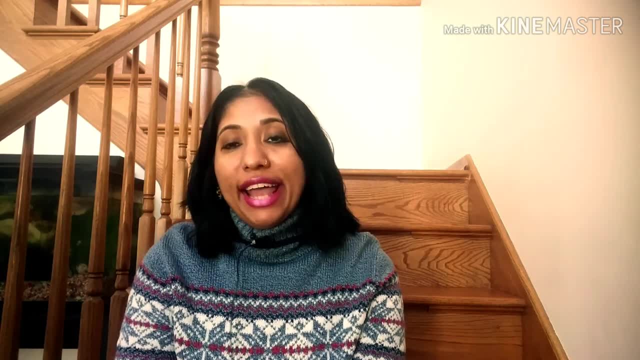 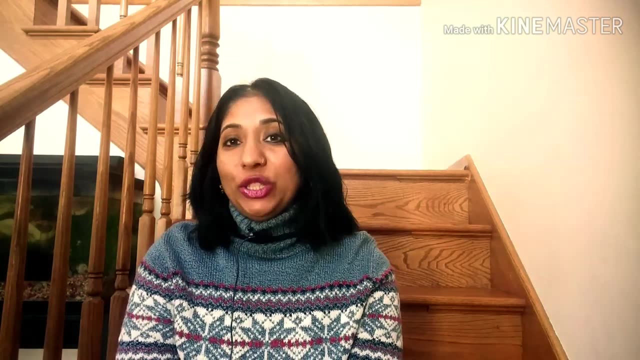 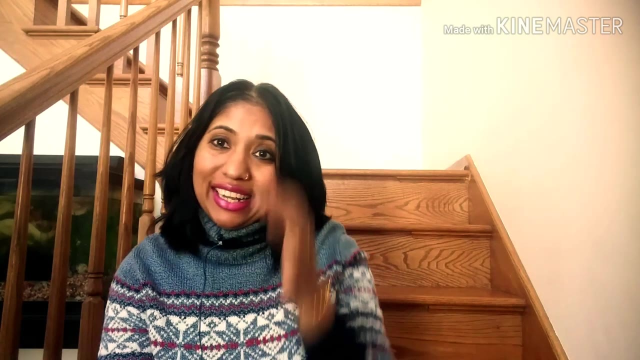 most of them are educated but they are more skill-oriented. Countries, government promote, you know government assist with their education and it's not that very expensive. So most of if you go to any eastern countries you know it's really hard to find a person without a minimum of. 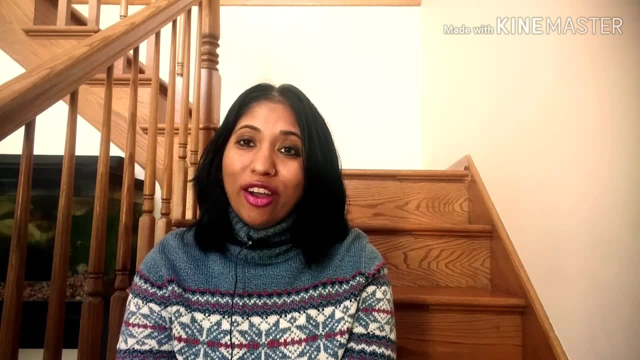 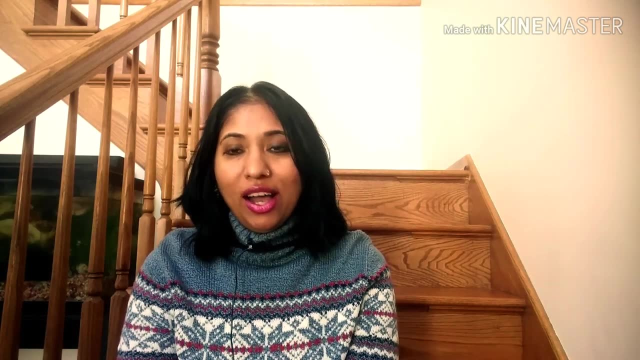 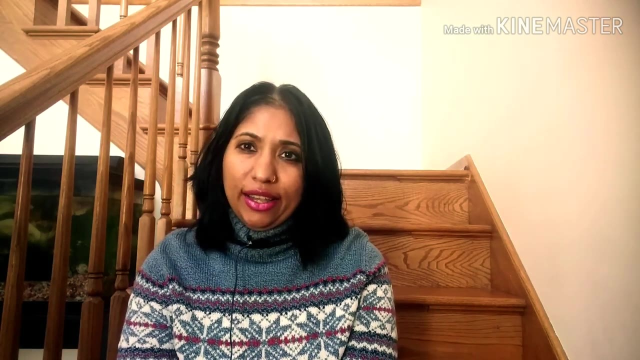 bachelor's degree, You will see more doctors, engineers and scientists. Most of them are from. majority of the people are from eastern countries, because we give much importance to education. Western countries, western countries, people are more skill-oriented. You know, they don't mind. 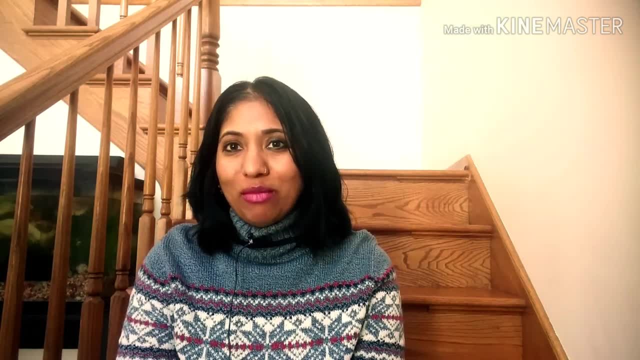 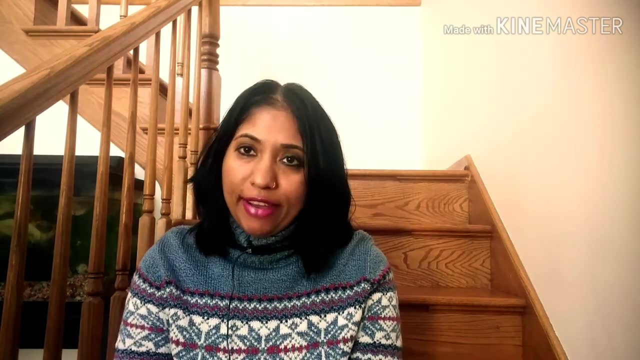 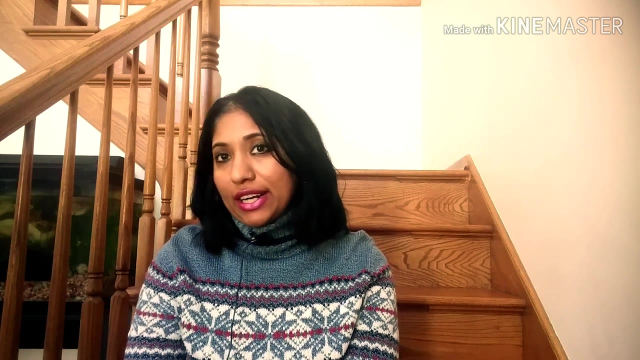 to take a small-scale job and you know some of them just stay at the same job forever and you know it's a little bit different that way. Education, education is very important, The only thing with the eastern culture. since most of the third world country. we are poor, So we had to go. 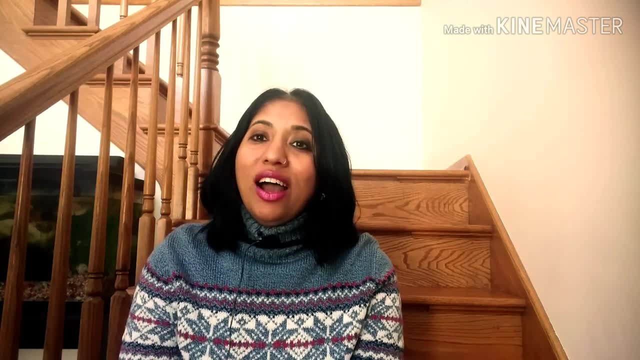 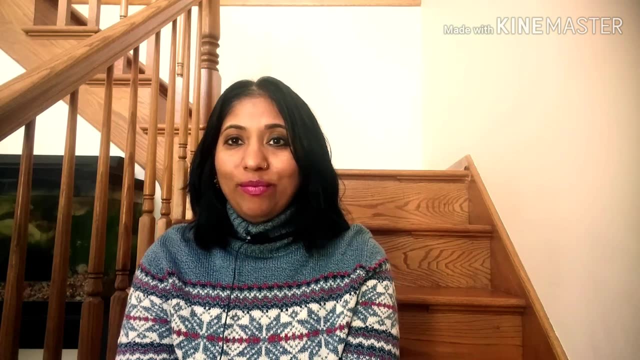 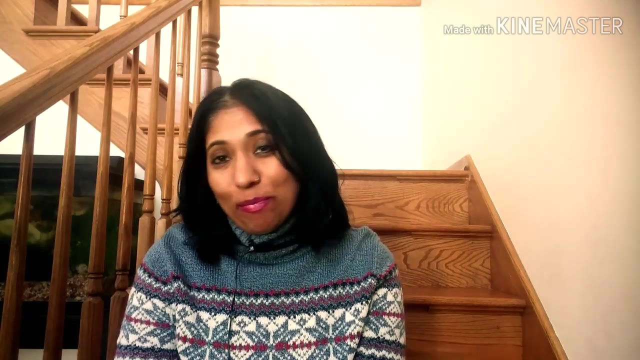 to other countries to get a better job and better living. Eastern countries people are all. another difference with the eastern culture is they are very respectful, They take care of their parents. they, you know- they rarely send people to nursing homes, Unlike western culture, people are busy. 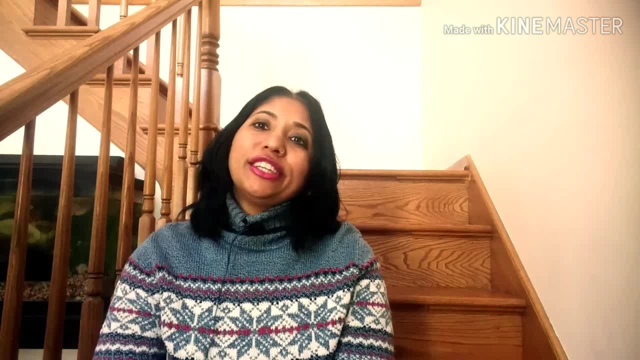 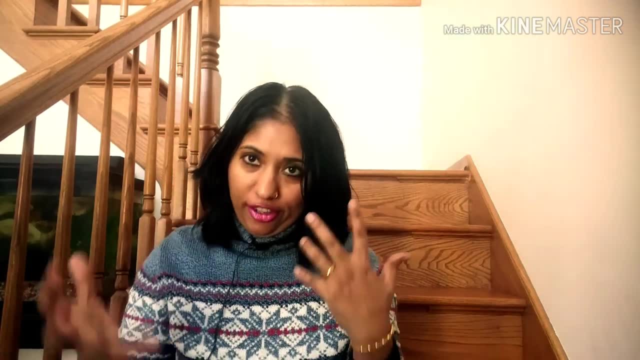 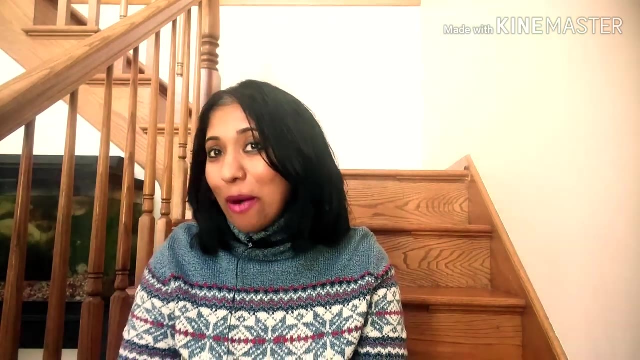 with their own life and most of the time they don't have, you know, time to take care of their elders. I mean, you know they are more, you know, independent, self-sufficient. I get it. you know, with the busy lifestyle here we don't have much time for it. A major difference between 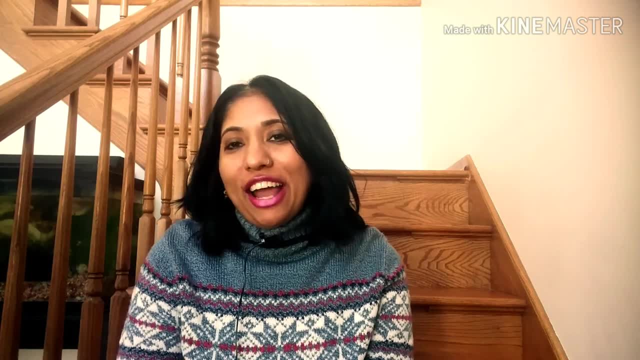 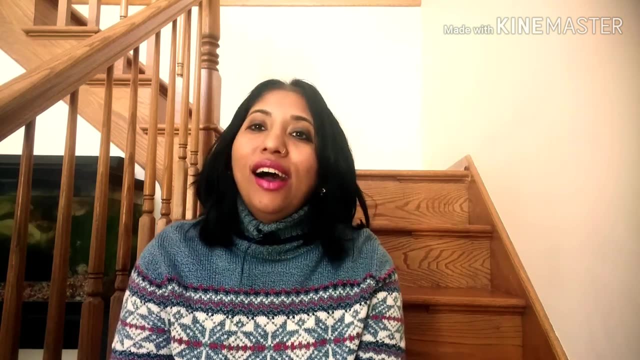 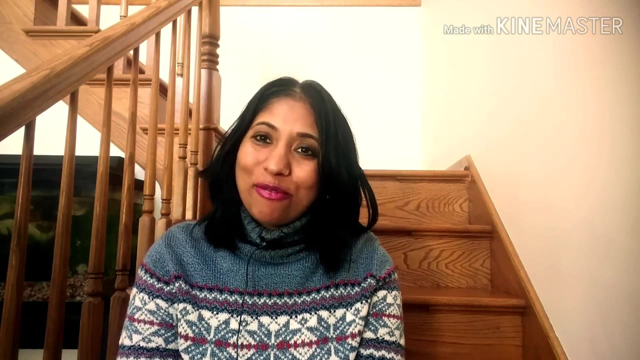 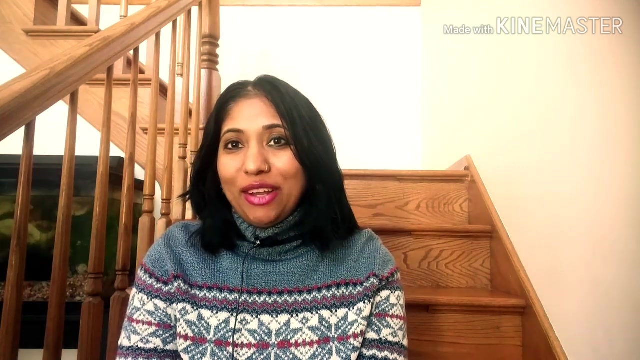 eastern culture, romantic life, Eastern culture, it's really hard to say a person say I love you to their partner. They may not say vocally, but they express through their action. Western culture is totally different. They, they are more vocal about it, you know, and the more romantic people. 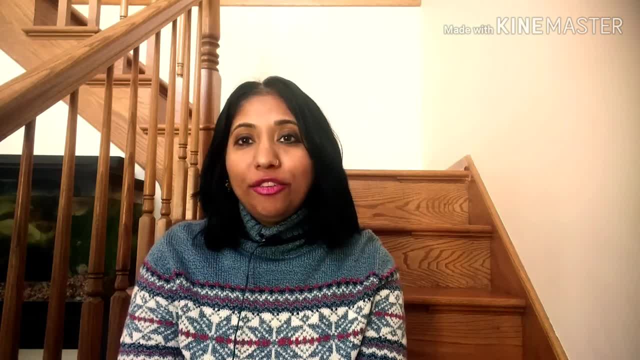 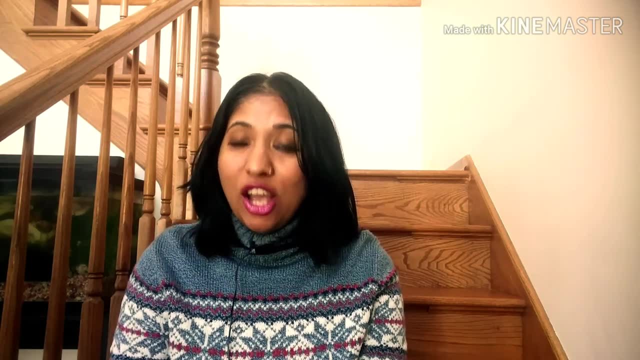 in general, Eastern culture. if you look at Western culture, it's very different Western culture if you get married- Eastern culture- you just don't get marry a person just for love. You look at their financial, social, economic as well as educational background and the job you know. 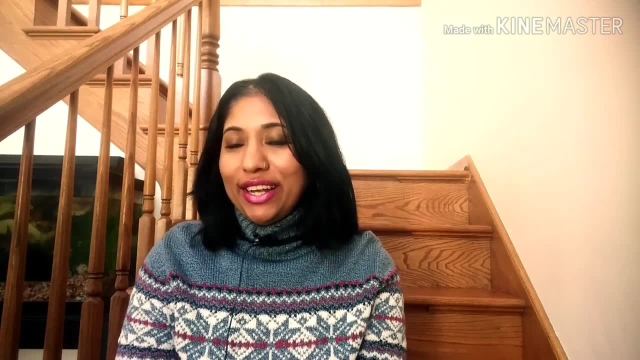 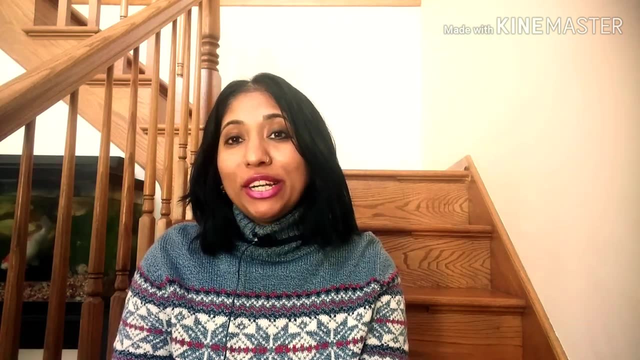 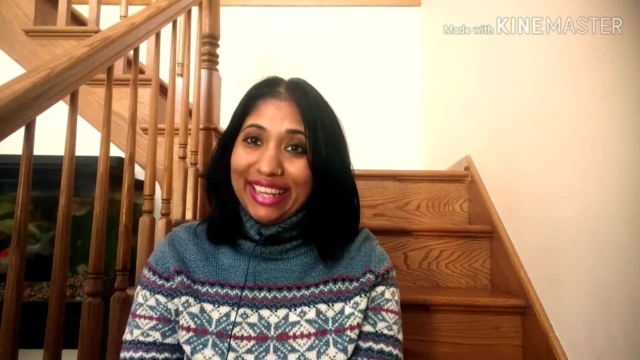 what type of job they are doing and everything That's very important in the eastern culture, Western culture, you, you might get married to a poor person for love. You don't think about as long as love can satisfy. you don't think about any other things: Economic, social, educational background. 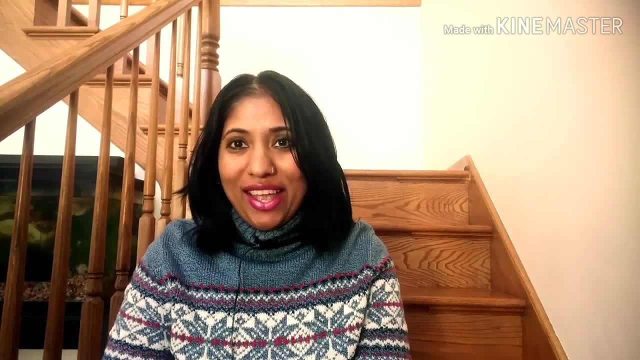 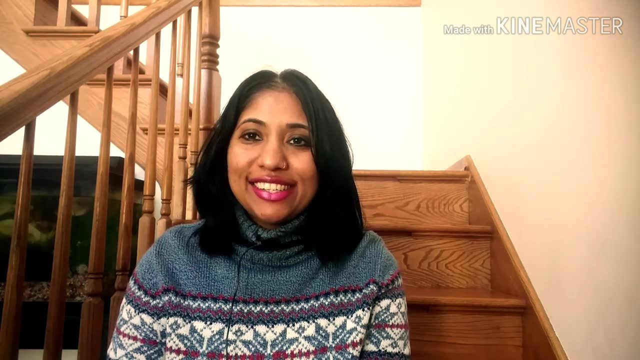 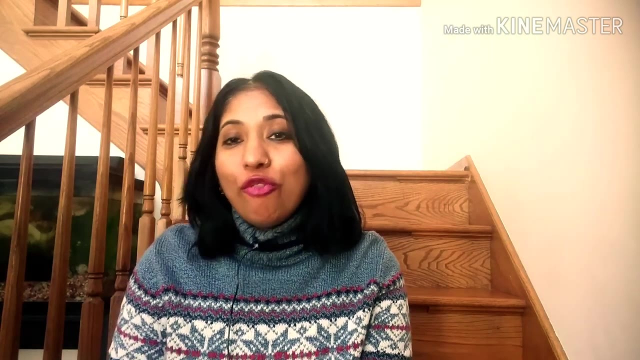 as long as love can satisfy, you are happy. That's a good thing too. I'm with them on that. Another difference between Eastern and Western culture is Eastern culture is more systematic, slow pace. Western culture is very fast forwarding and you go and get you know that type of thing. 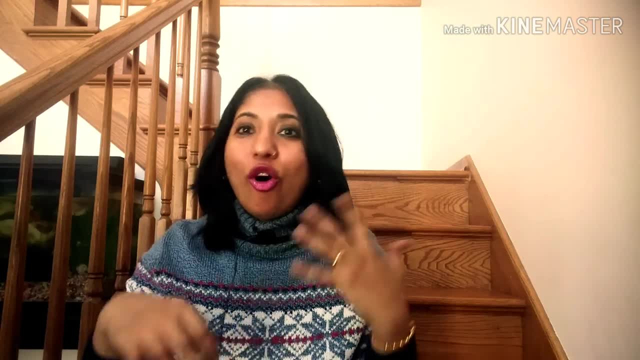 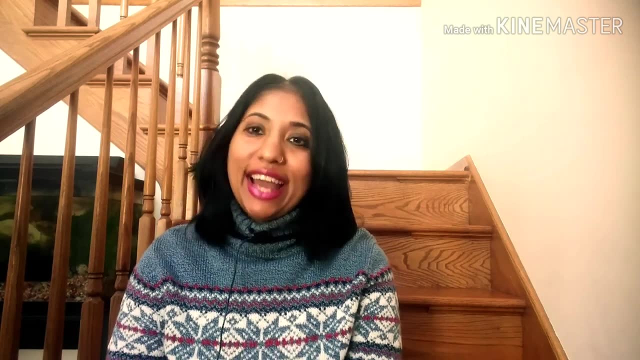 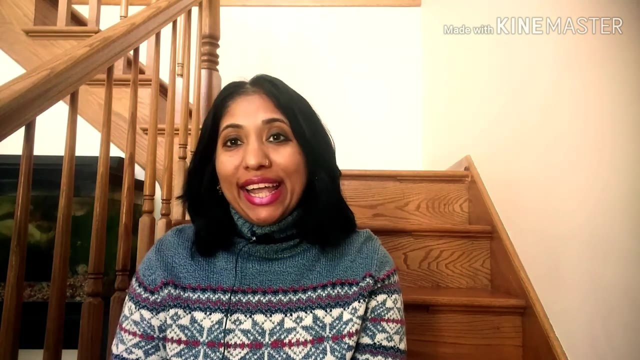 you know you go and get accomplished more stuff. It's more fast forward. you know it's just a busy life. Parents in Eastern- you know culture- think that they have an obligation to take care of their kids, obligation to make a decision in their kids' life. So they help them with education and you. 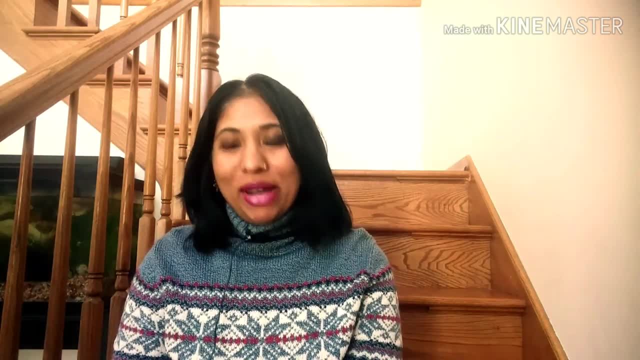 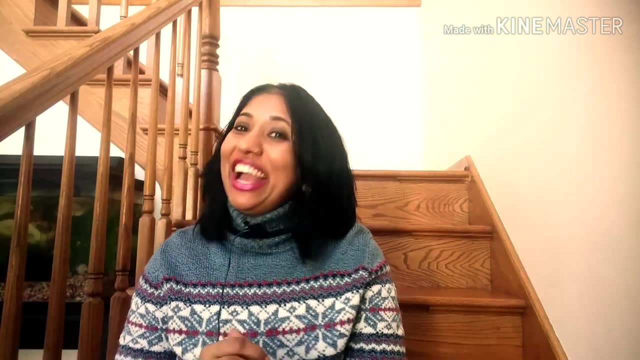 know their homework and try to get, help them to get a job and stuff like that. They are more involved in kids' culture. I'm I had to admit that I'm one of them. you know, I can tell kids, you know. 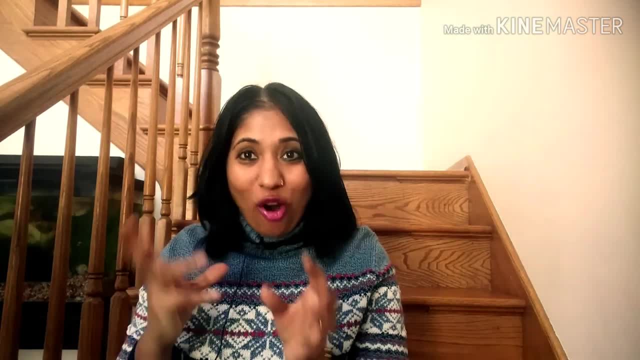 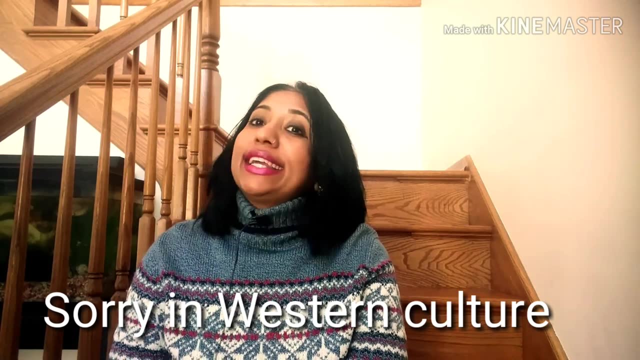 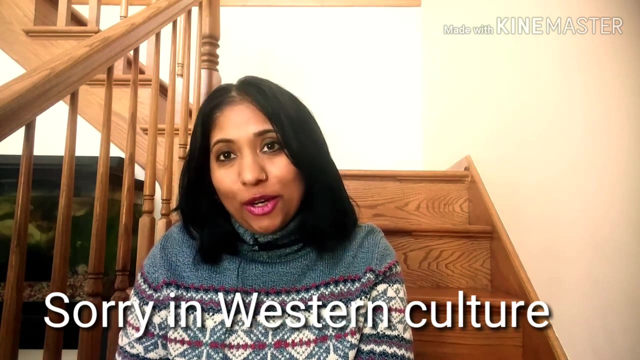 study more and, you know, get more accomplished. I can constantly push the kids, I had to admit on that- And Eastern culture. parents give them a choice. Kids can choose their own life and they can make their own decision about their life. That's a good thing and a bad thing. Good thing: 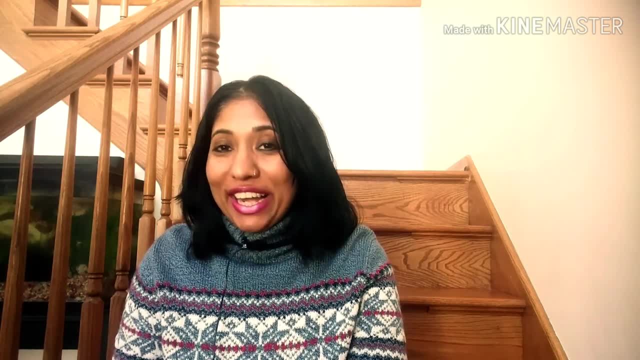 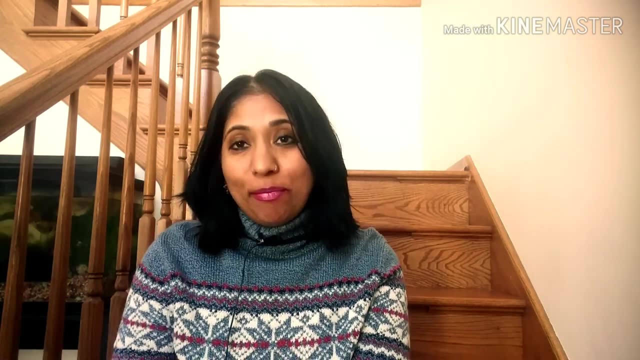 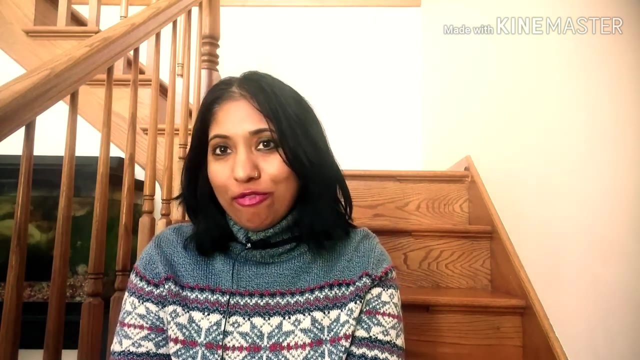 is that kids are not pushy. So kids can decide to do whatever they want and it's their freedom. Another thing with the financial aspect: Eastern people are more conservative with their money. You know, even if they lose the job they'll be okay for a year at least. They have that, you know. 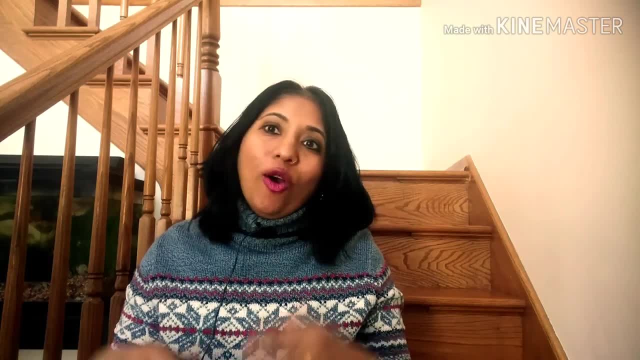 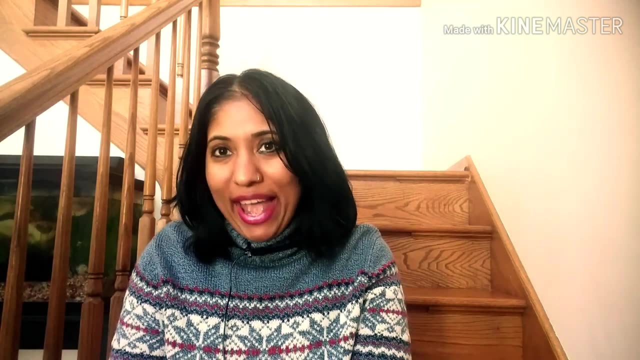 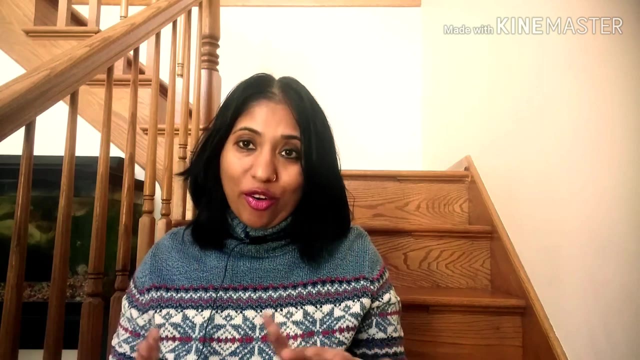 backup fund to survive. You know they already accomplished their. you know, at the around at 30 they accomplish, they get married Most of the time they have. they started to have their family. They already have, you know, their own home and you know they are pretty accomplished by the age. 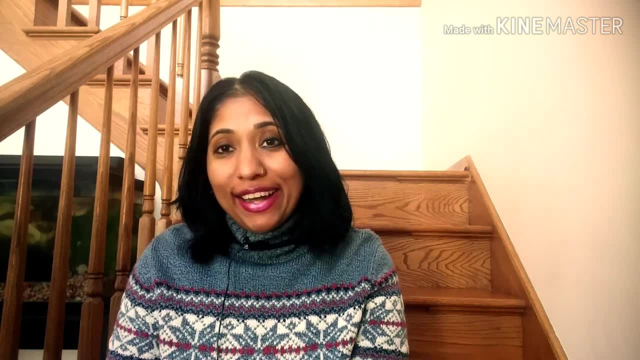 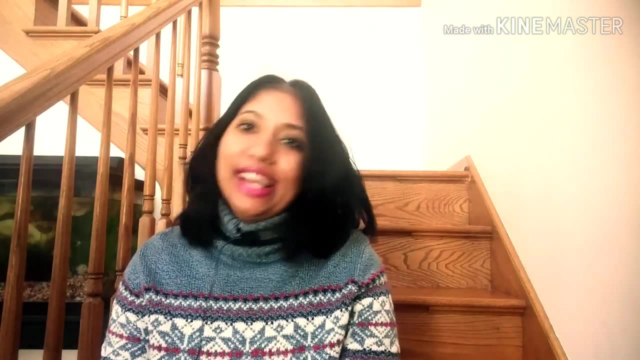 of 30. Western people: they are more fun loving. you know they don't think about their life. you know, till they are 40s. Then you know, even if you get married before age of 40, you are still. 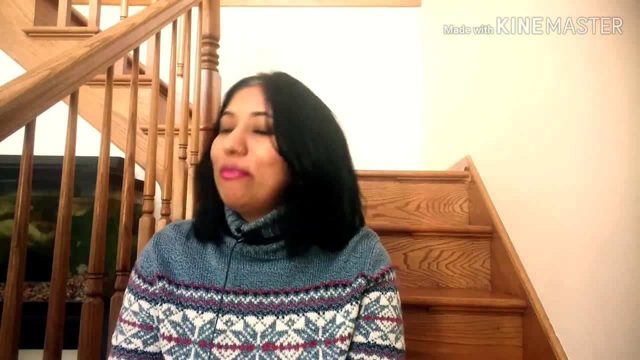 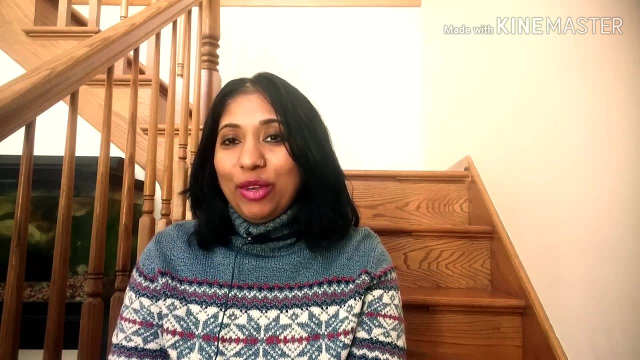 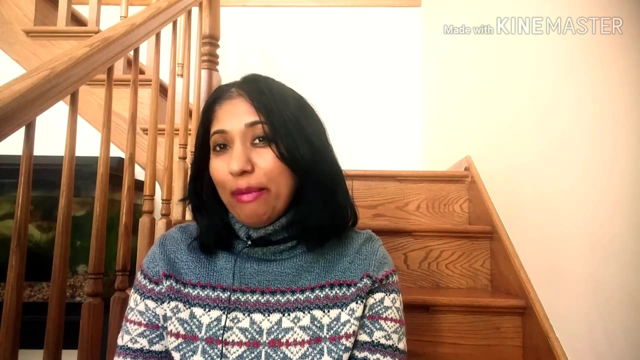 they get to know each other and you know taking their time and stuff like that, They don't give much importance to their financial situation, you know, until something- Castro, you know something bad happens. I had to admit that's one of the bad thing about Western culture. I had to admit that, Please. 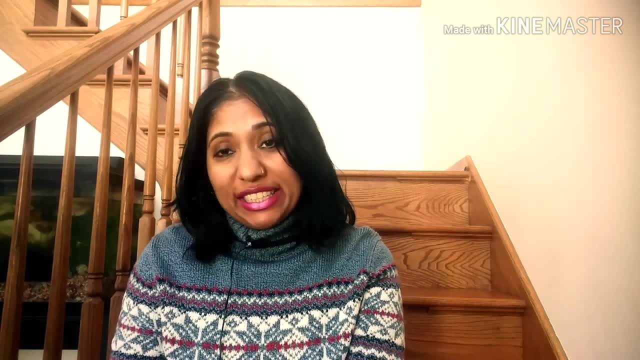 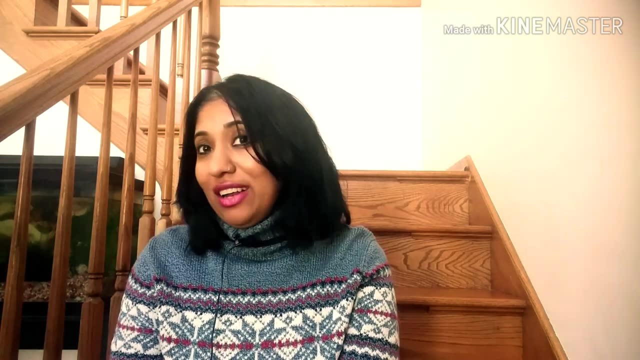 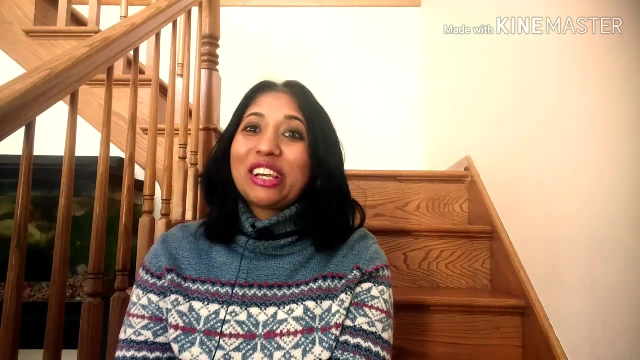 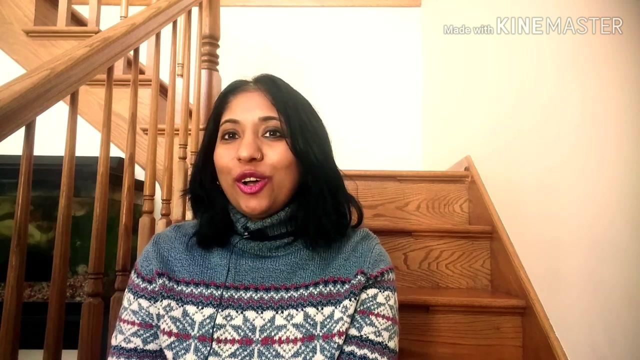 don't get offended with that. You know, majority of the Western people live paycheck to paycheck, which can be a bad thing. You know, when, like recent episode, like federal shutdown happened and people has to depend on the social service program to, you know, survey their day to day expense. So Eastern culture they are. 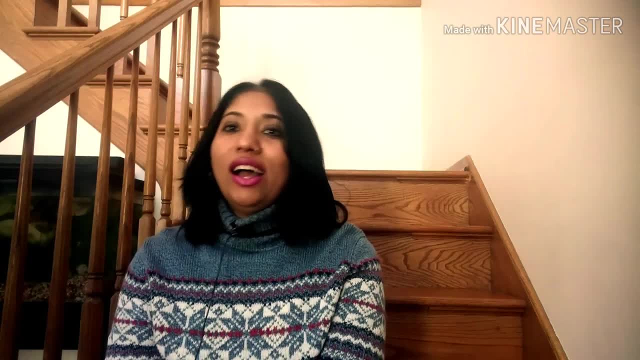 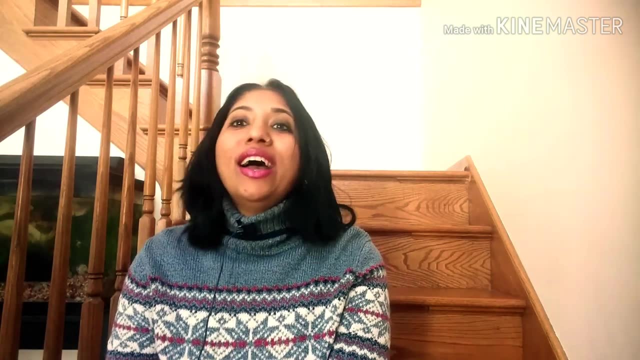 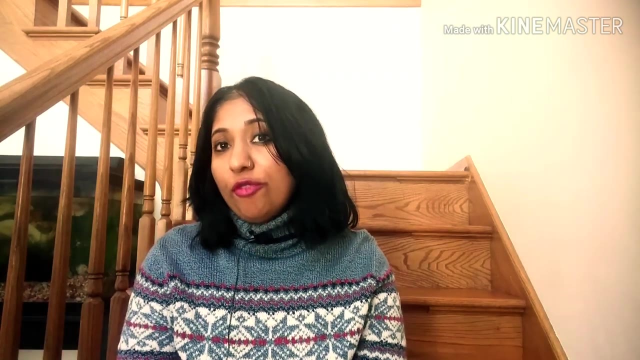 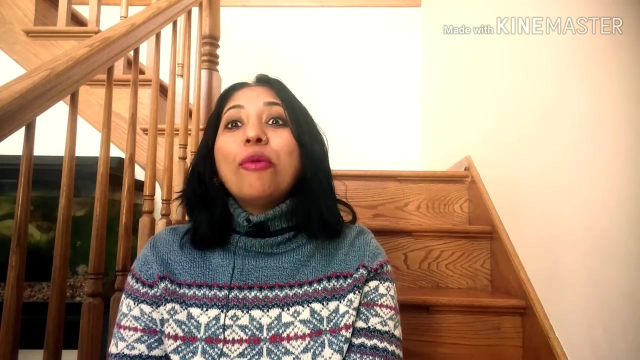 very conservative. they don't waste their money for unnecessary things And financially they are more secure compared to Western. you know people. Another is an additional tip I'm giving you from my years of experience. for me, it's not about how much money you make. it is how much you save, Even if 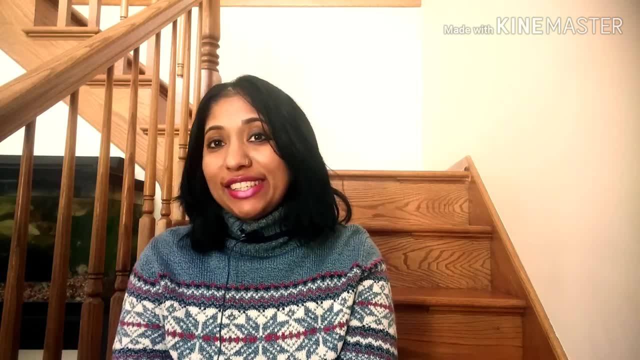 you make only 1000 dollars a month. as long as you can save a hundred dollar, you know. then if you make, if you make $5,000 a month, then if you don't save any, anything, any, if you're looking for the next 100, Christ, come in now. do you want anything new in the sector? do you want to give something for my salary, which I like individual income? do you want to give twelve thousand dollars a month? 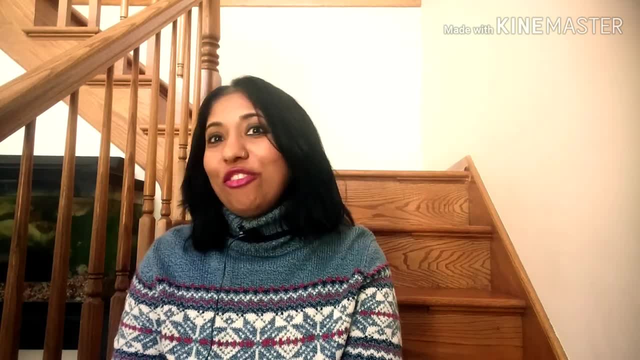 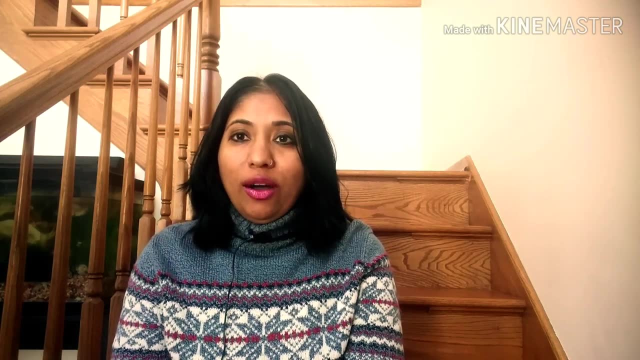 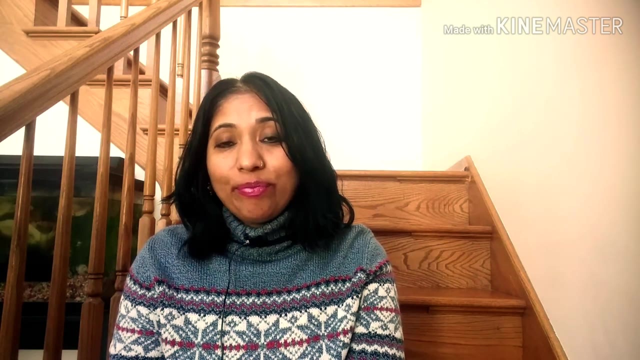 five thousand dollars a month, then if you don't save any, anything, any- if you are looking for the next 500, then there is a pressure and paycheck to come around. so it's not about how much you make, it's about how much you save. if you have different ideas, you know, among between Eastern and